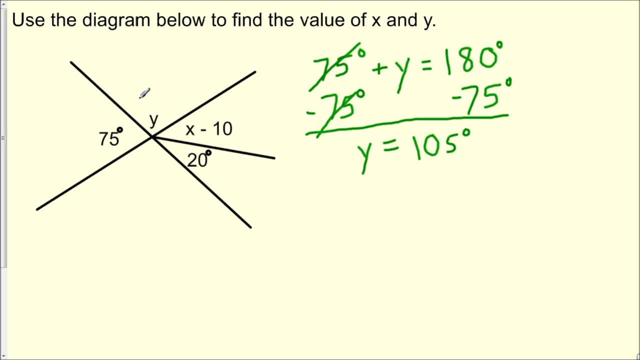 set up the equation. Now that we know that y is 105 degrees, we could focus on another straight angle. We have this 105 degree angle, this angle x minus 10, and this angle of 20 degrees, But together these three angles build another straight line. So what we could do is we could add these: 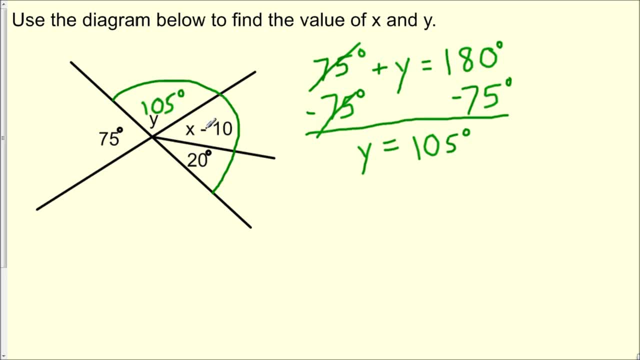 three angles together and set that equal to 180 degrees. So what equation we could set up. We could set up: 105 degrees plus x, minus 10, plus 20 degrees equals 180 degrees. And now, just to be formal, we'll put a degree symbol on it. We're just going to put a. 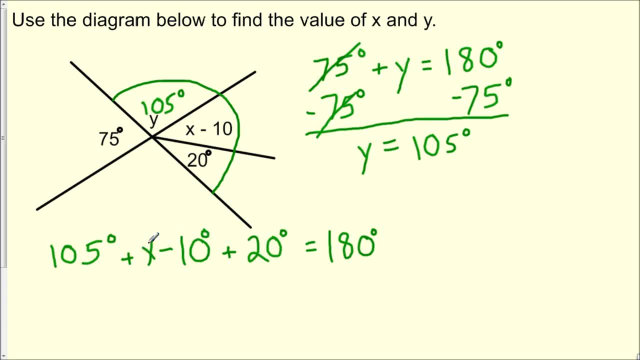 1., 2., 3., 4. around 10, but this is really x degrees minus 10 degrees. but the symbols are important. so now what we could do is we can combine like terms. we have 105 minus 10 plus 20. well, 105 minus 10 is 95, and 95 plus 20 is 115. so now what we could. 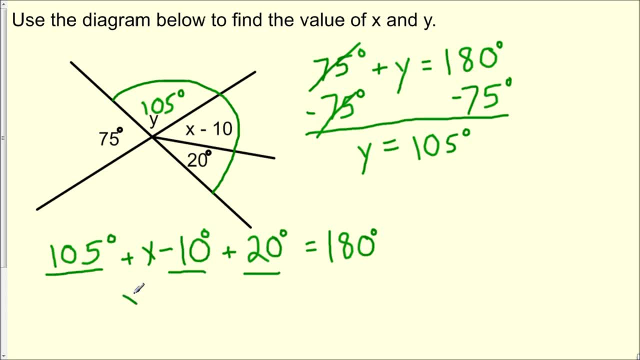 set up is: we have: X plus 115 degrees equals 180 degrees. so now to solve for X, all we need to do is subtract 115 degrees from both sides of this equation, and now we note on the left hand side: 115 degrees minus 115 degrees cancels. 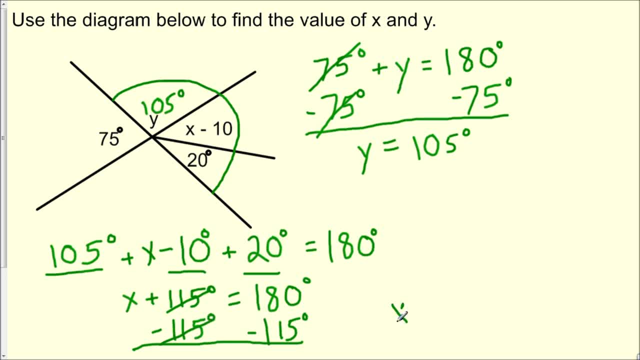 leaving us with X equals, and now, 180 degrees minus 115 degrees is equal to 65 degrees. so the value of why we have 105 degrees and the value of X: we have 65 degrees. but now remember, if this were a test, it's always a good idea to check.